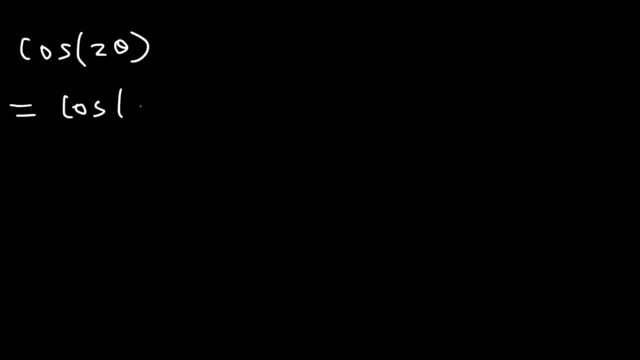 So cosine 2 theta is cosine theta plus theta, And we're going to use the sum and difference formulas for cosine Cosine alpha plus beta, that's cosine alpha, cosine beta minus sine alpha, Sine beta. So then this is going to be cosine theta times cosine theta, where alpha and beta are both theta minus sine theta times sine theta. 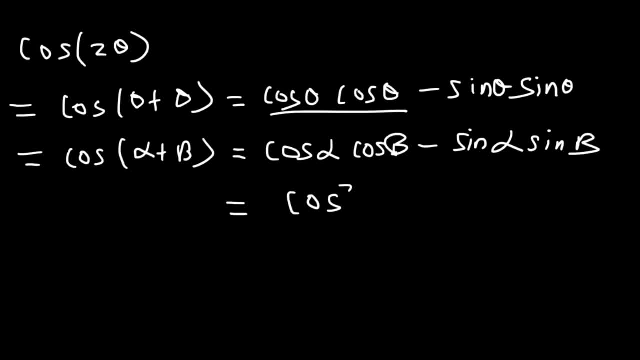 Now cosine times cosine, that's cosine squared. And sine times sine, well, that's going to be sine squared. So now we have the double angle formula for cosine 2 theta. So cosine 2 theta Is equal to cosine squared minus sine squared. 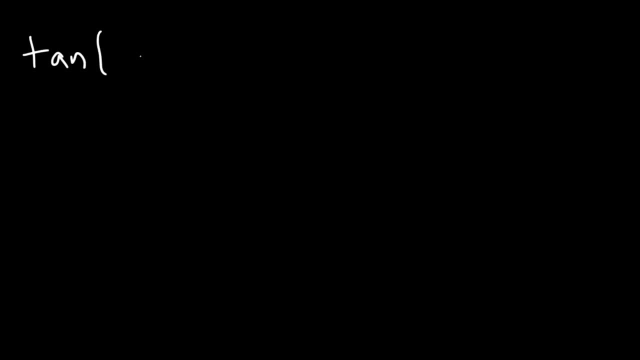 Now let's move on to tangent. We know that tangent alpha plus beta is equal to tangent alpha plus tangent beta divided by 1 minus tan alpha, tan beta. So now let's find the value of tangent theta plus theta. This is going to be equal to: 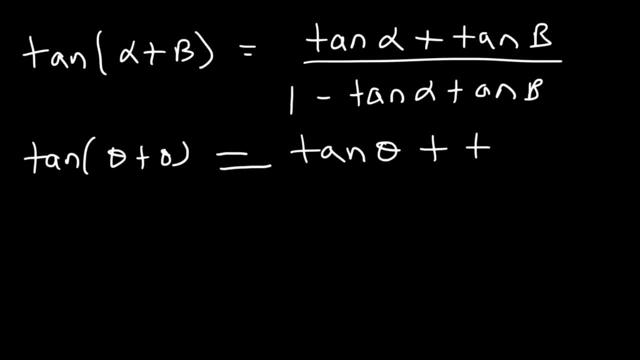 Tangent theta plus tangent theta, which is all divided by 1 minus tan theta times tan theta. So tan theta plus tan theta, that's 2 tangent theta, And on the bottom, tangent theta times tangent theta, that's equal to tan squared. 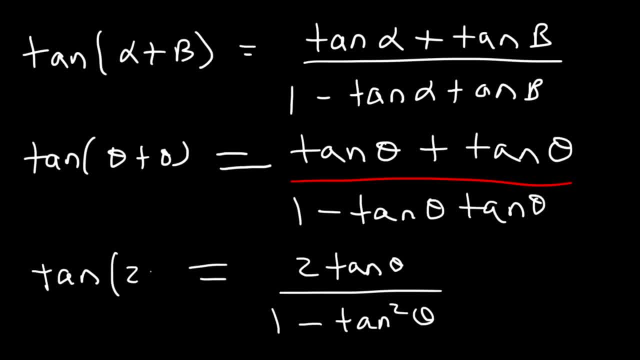 So all of this is equal to tangent, theta plus theta, which is 2 theta. So here we have the double angle formula Of tangent. So make sure you write down those three formulas, because we're going to use them soon. Now let's say that sine theta, 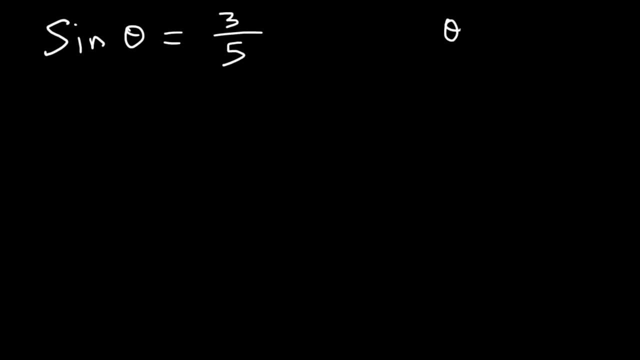 Is equal to 3 divided by 5.. And theta Is between 0 and pi over 2.. With this information, Find the values of sine 2 theta, cosine 2 theta and tangent 2 theta. So the first thing we need to do is draw a right triangle. 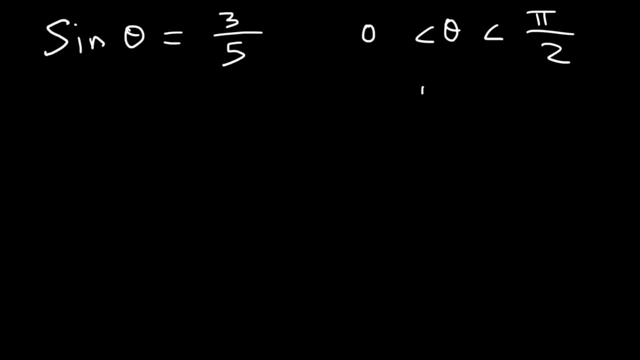 And notice that theta is in quadrant 1.. So that's where we're going to draw the right triangle. So here's the angle. theta, in its standard position, Sine, is opposite divided by hypotenuse. Now this is the 3,, 4,, 5 right triangle. 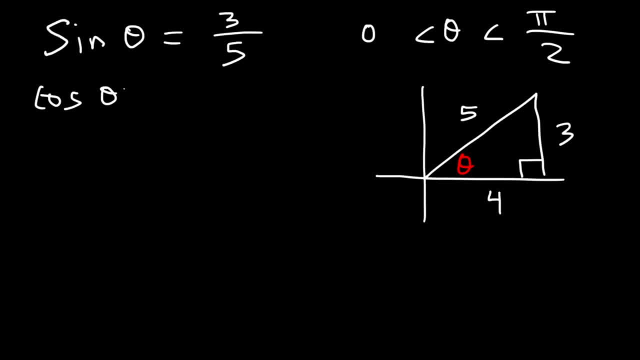 So now we can find cosine, Cosine, theta. according to SOHCAHTOA, it's equal to the adjacent side divided by the hypotenuse, So that's 4 over 5.. So recall that 4 is adjacent to theta. 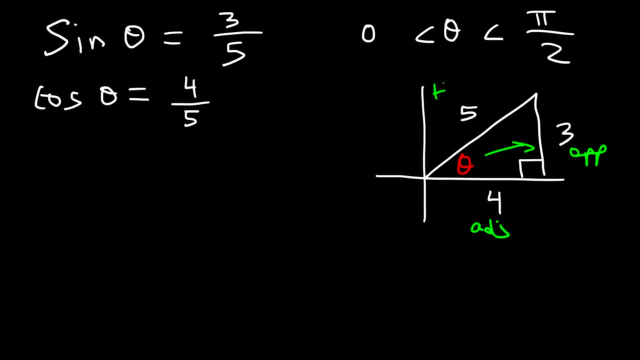 3 is opposite to theta And 5 is the hypotenuse. It's the longest side of the three sides of the triangle. Now we need to find tangent theta. Tan theta is equal to the opposite side divided by the adjacent side. 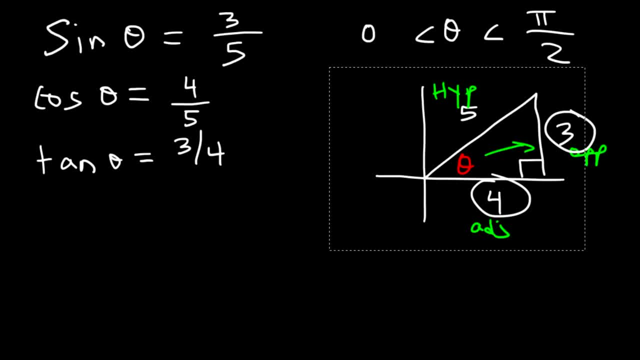 So in this case it's 3 divided by 4.. Now that we have sine cosine and tangent, We can solve everything. I know I'm going to need more space, so I'm just going to rewrite tangent on this side. 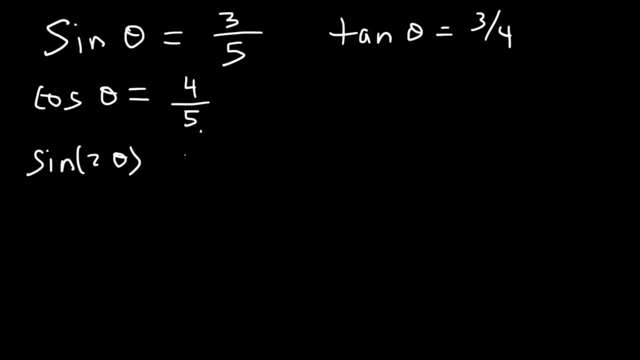 Now let's find the value of sine 2 theta. Sine 2 theta is equal to 2 sine times cosine theta. Now we have the value of sine. Sine theta is equal to 3 divided by 5. And we have the value of cosine. 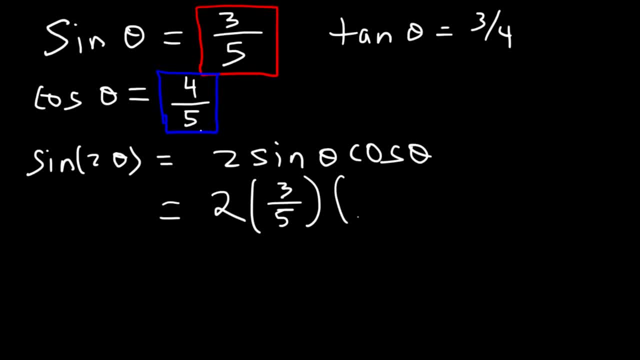 Cosine theta is 4 over 5.. So all we got to do is just plug this in to the equation. So 2 is the same as 2 over 1,, by the way. So we need to multiply 2 times 3,, which is 6 times 4.. 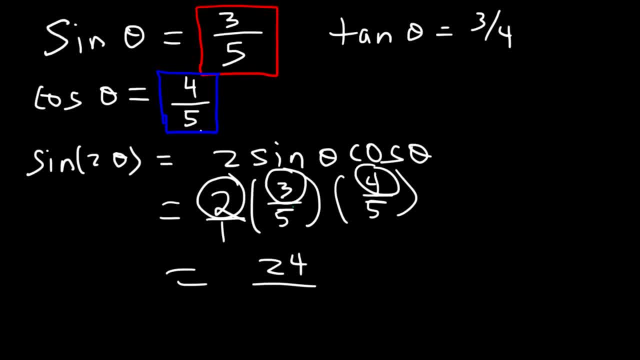 That's 24.. And then let's multiply the numbers on the bottom: 5 times 5 is 25.. That's 4.. That's 5.. That's 6.. So sine theta, or rather sine 2 theta, is equal to 24 divided by 25.. 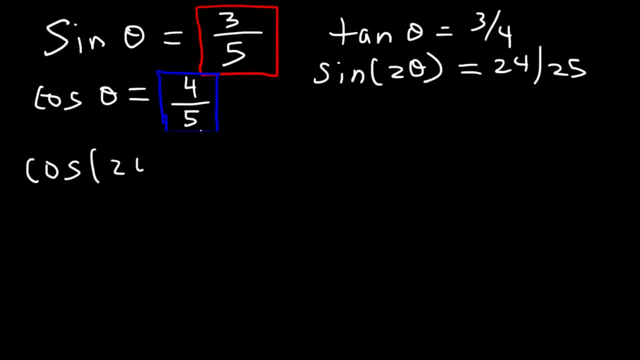 Now let's find the value of cosine 2 theta. So let's use the formula cosine squared minus sine squared, Cosine is 4 divided by 5.. Sine is 3 over 5.. 4 squared is 16.. 5 squared is 25.. 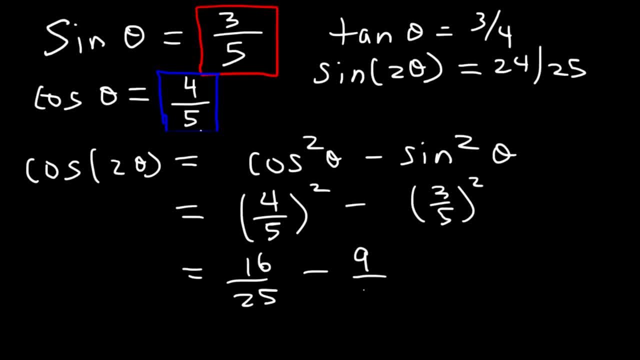 3 squared is 9.. And 16 minus 9, that's 7.. So cosine 2 theta is 7 divided by 25.. All right, All right. Next we need to find tangent. There's two ways you could find tangent 2 theta, and I'm going to show you both. 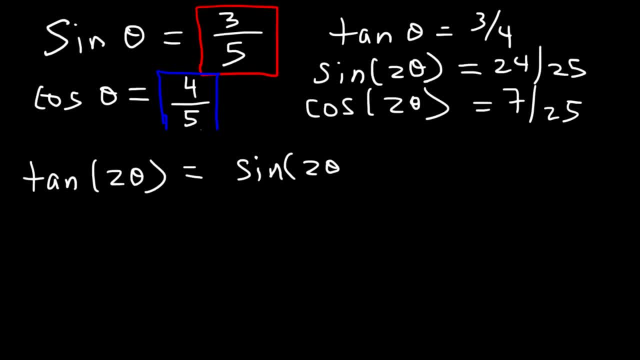 The first method is to use this formula. You know that tangent is sine divided by cosine. This is the quotient identity, so let's plug in everything. So sine is 24 over 25, and cosine 2, theta is 7 divided by 25.. 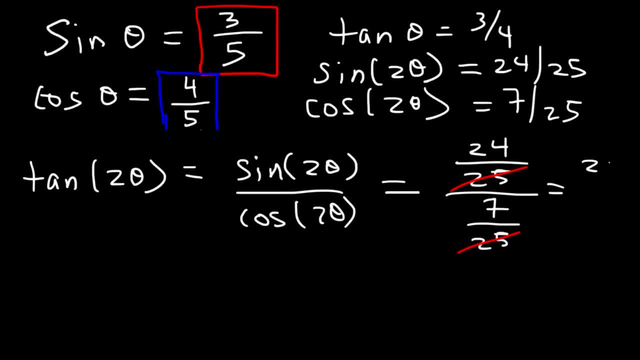 We could cancel the 25s, and so tangent 2 theta is 24 over 7.. Now let's see if we can get that same answer using another formula. So let's write it here: tangent 2 theta is 24 over 7.. 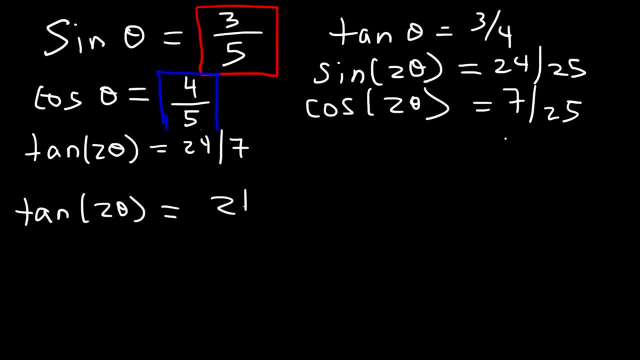 Now we can also use the fact that tangent is 2 tan theta divided by 1, minus tangent squared. So we have tangent theta which is 3 divided by 4.. So 2 times 3 fourths. What is that? 2 times 3 fourths is 6 fourths. 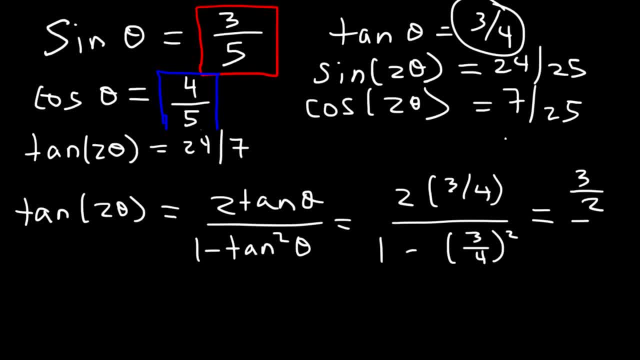 6 over 4 reduces to 3 over 2.. And 3 squared is 9,, 4 squared is 16.. Now, at this point, I'm going to multiply the top and the bottom by 16 to get rid of all. 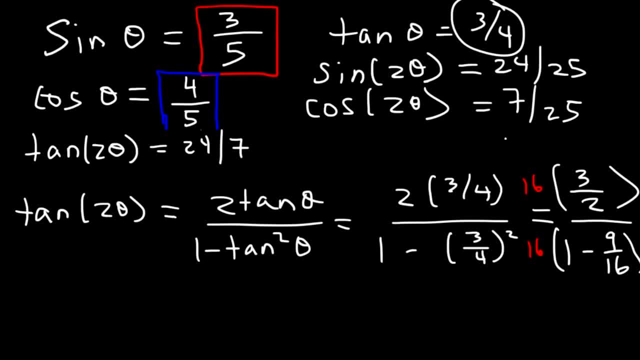 fractions. So what is 16 times 3 divided by 2?? It might be easier to divide first. 16 divided by 2 is 8 times 3.. That's 24.. On the bottom we have 16 times 1, and that's 16.. 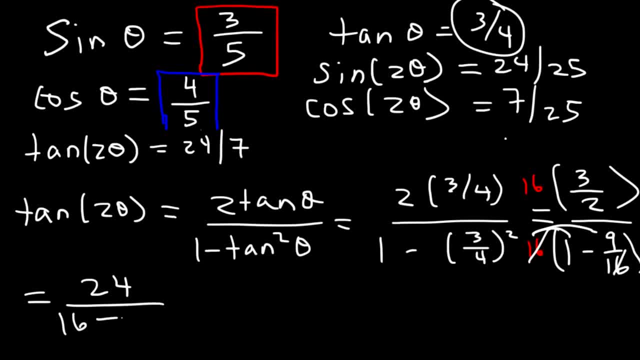 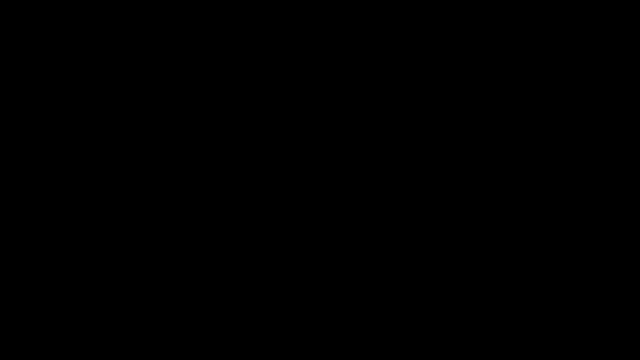 And then 16 times 9 over 16. These will cancel and we'll just get negative 9.. 16 minus 9 is 7.. So this will give us the same answer of 24 divided by 7.. But I think the first method is a lot easier than the second one. 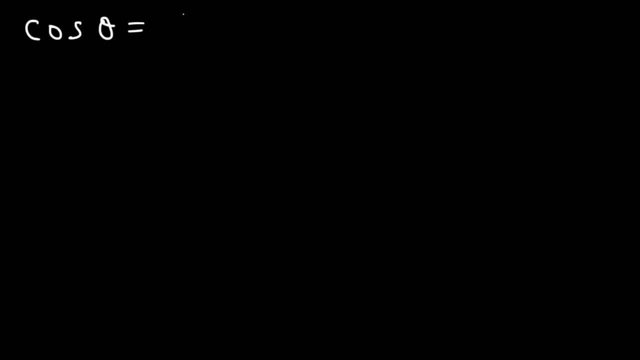 Here's another example that you could try. Let's say that cosine theta is equal to 5 divided by 7. That's 4 divided by 13. And theta is in between 3 pi over 2 and 2 pi. Go ahead and find the other values. 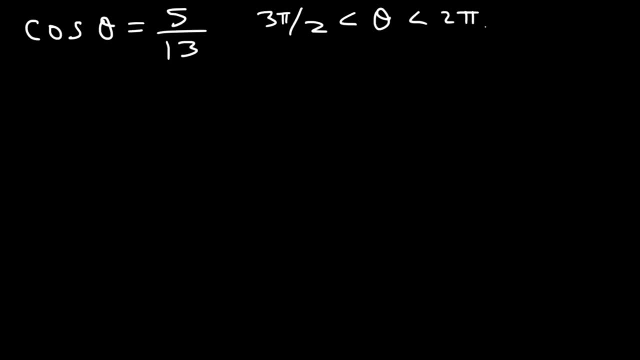 Sine 2 theta, cosine 2 theta and tangent 2 theta. Find the double angles of those three functions. Now the first thing we need to do is draw the triangle. The triangle exists in quadrant 4 because theta is between 270 and 360. 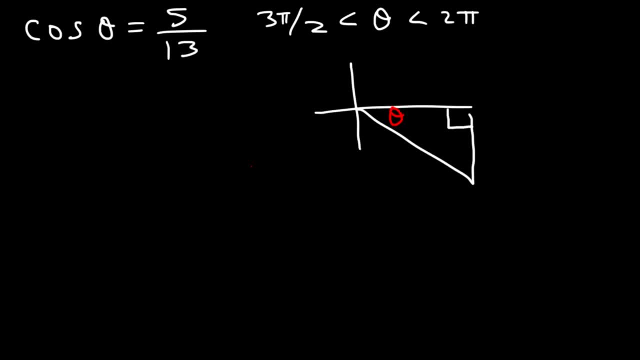 Let's draw the triangle. So here's the angle theta. Now we know that cosine is equal to the adjacent side divided by the hypotenuse. So this is 5, and that's 13.. This is the 5,, 12,, 13 triangle. 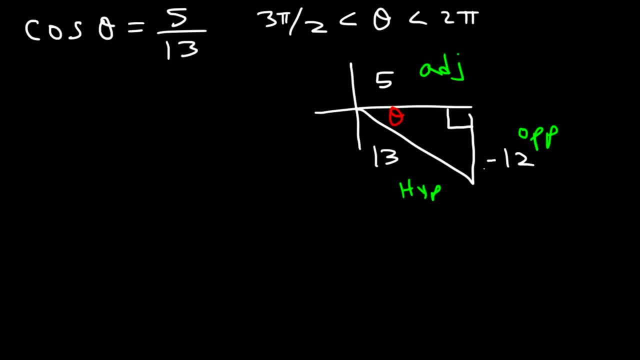 Now y is negative in quadrant 4, so this is going to be negative 12.. Now we need to find sine theta. Sine theta is opposite divided by hypotenuse, And that is not hypotenuse. The hypotenuse is 13.. 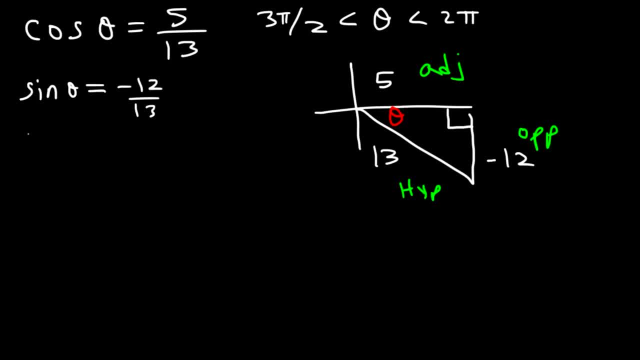 So sine theta is negative 12 over 13.. Tangent theta, that's equal to opposite over adjacent, So that's negative 12 over 5.. Now let's see if I can rewrite everything on top to conserve space. So now let's start with sine 2 theta. 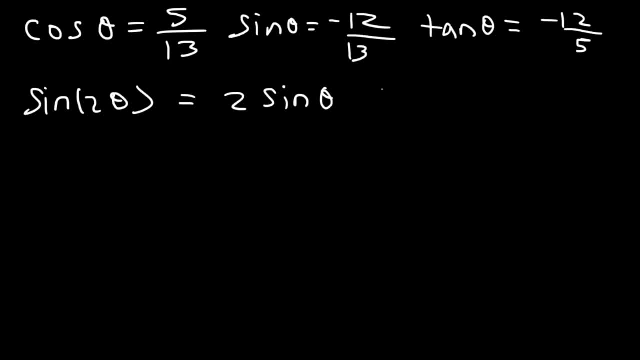 So this is equal to 2 sine theta multiplied by cosine theta. Now we have that sine is negative 12 divided by 13.. And cosine is 5 divided by 13.. So 2 times 5 is 10.. 10 times negative 12.. 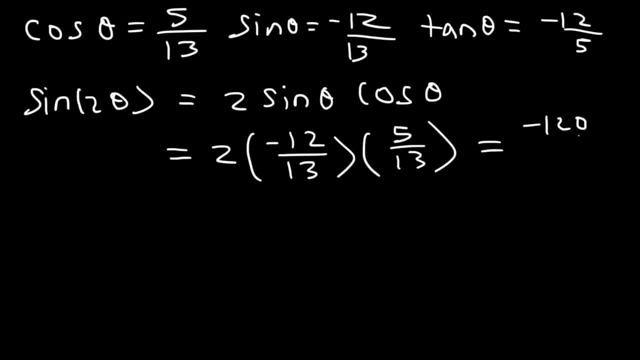 That's negative 120.. 13 times 13 is 169.. So here's the value of sine 2 theta. It's negative 120 over 169.. Now let's look at sine 2 theta. So sine 2 theta is negative 12 over 169.. 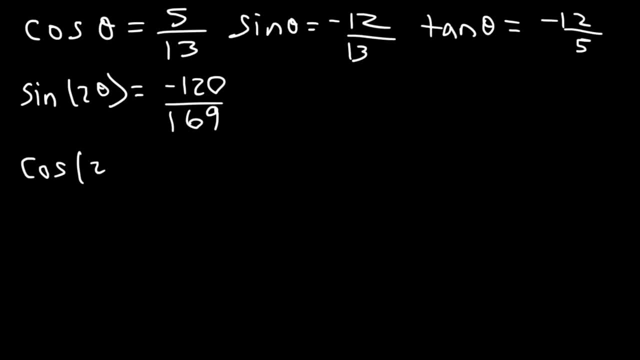 So sine 2 theta is negative 12 over 169.. Now let's work on cosine 2 theta. So let's use the formula cosine squared minus sine. squared Cosine is 5 divided by 13.. Sine is negative 12 divided by 13.. 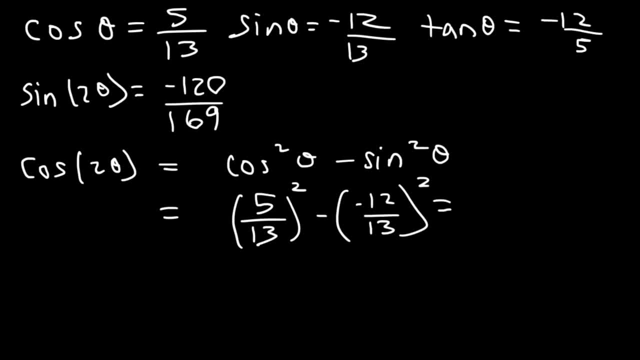 And we've got to square each one. So 5 squared is 25.. 13 squared is 169.. 12 squared is 144.. But it's a negative in front. So negative 12 squared, that's positive 144 times the negative on the outside. 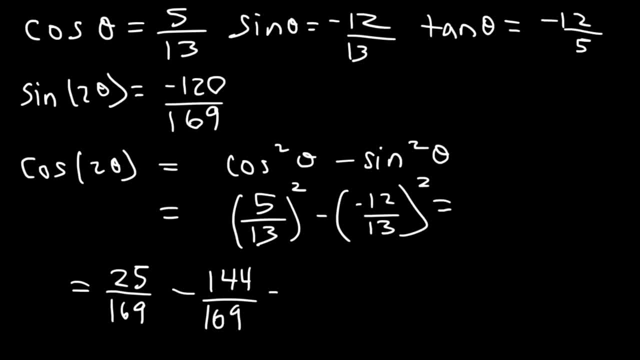 So it's going to be negative 144 over 169.. So if we subtract 25 by 144, this will give us negative 119.. And so that's the value of cosine 2 theta, Which I'm going to write it right here. 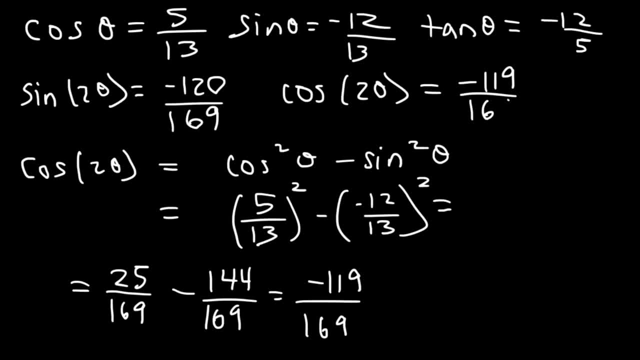 Now let's find the value of tangent 2 theta. So tangent 2 theta is equal to 2, I mean sine 2 theta divided by cosine 2 theta. So that's negative 120 over 169.. Divided by cosine 2 theta: 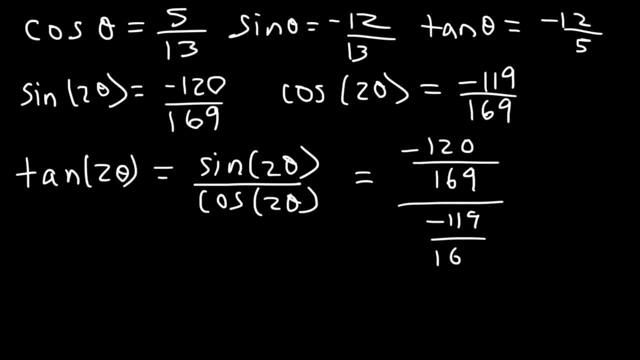 So that's negative 120 over 169.. Divided by negative: 119 over 169.. So we can cancel these two. The two negative signs will cancel, And so this is going to be positive 120 over 119.. And so that's it. 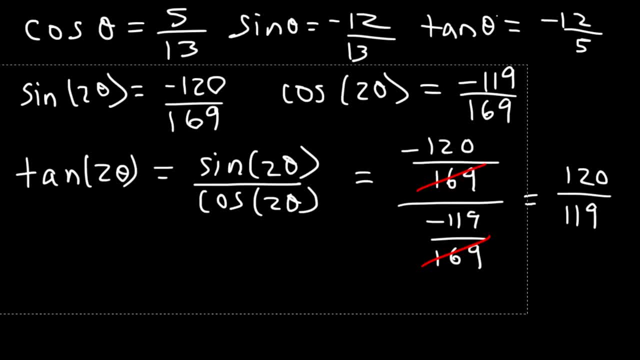 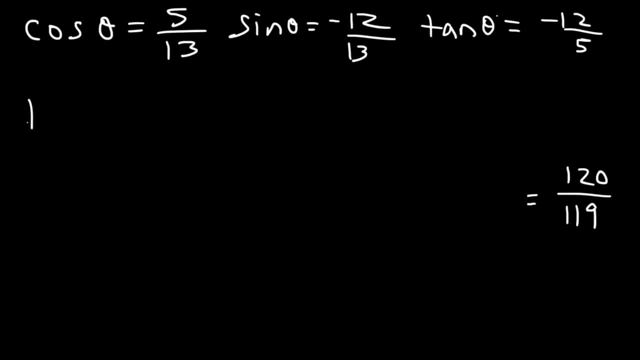 Now let's confirm our answer with the other formula So you can be familiar how to use it, Because sometimes the only thing you may have is just tangent. So tan 2 theta is equal to 2 tangent theta over 1 minus tan squared. 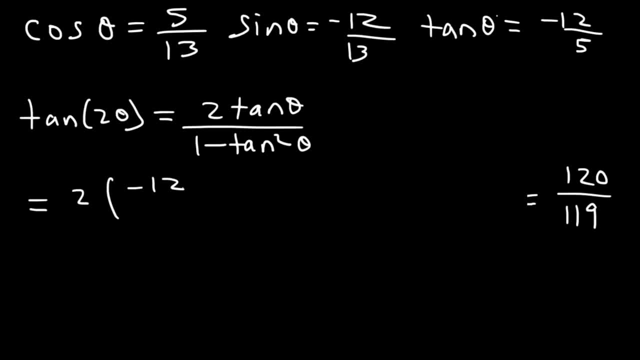 So using that formula we have tangent theta is negative 12 divided by 5. Divided by 1 minus tan squared, which is negative 12 over 5 squared, So 2 times negative 12, that's negative 24.. 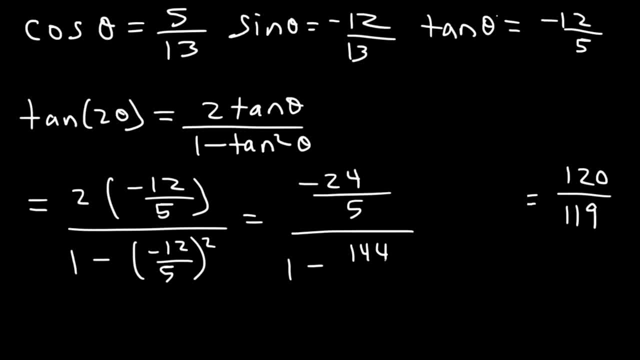 Negative: 12 squared is 144.. 5 squared is 25.. So I'm going to multiply the top and the bottom by 25.. 25 divided by 5 is 5.. And 5 times negative 24,. well, that's negative 120.. 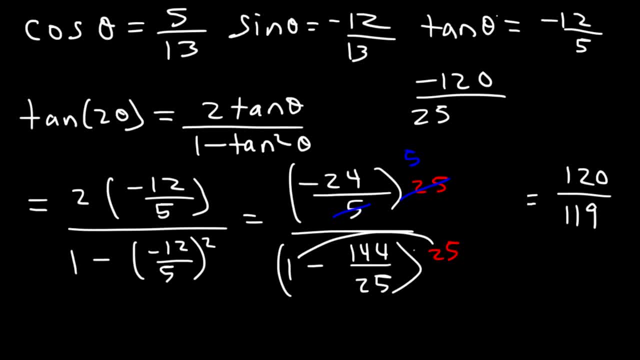 25 times 1 is 25.. 25 times 144 over 25, that's going to be negative 144.. 25 minus 144 is negative 119.. Two negatives will cancel to give you a positive result. So you get the same answer: 120 over 119. 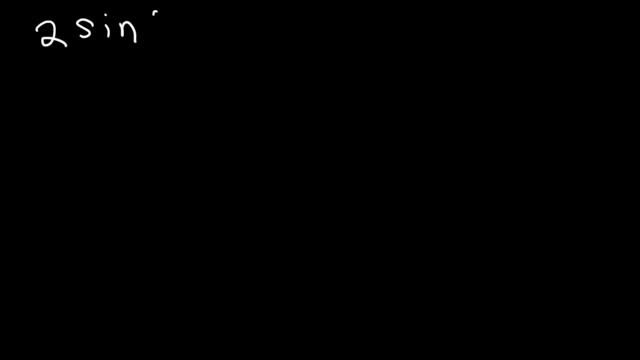 Now what would you do if you saw a problem like this: 2 sine 75 degrees times cosine 75 degrees. Find the exact value of that. Now we don't know the value of sine 75. However, we could use the double angle formula of sine to get the answer. 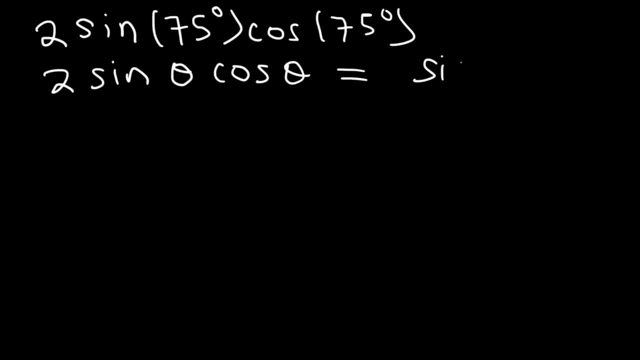 2 sine theta. cosine theta, we know, is sine 2 theta, So clearly we can see that theta is 75.. So this expression is equal to sine times or sine of 2 times 75 degrees, So that's 75.. 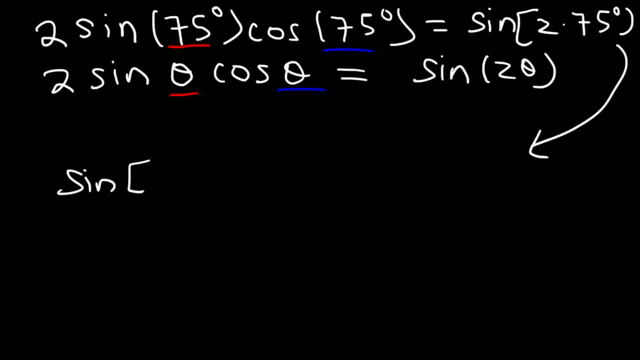 Which is equal to sine of 150 degrees. 150 has a reference angle of 30 degrees And according to the 30-60-90 triangle, sine 30 is opposite over hypotenuse. So that's 1: half And 150 is in quadrant 2.. 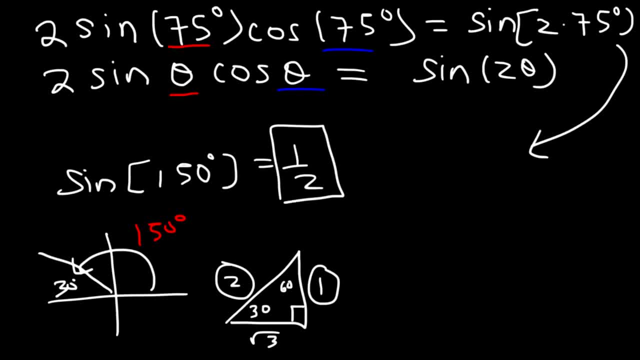 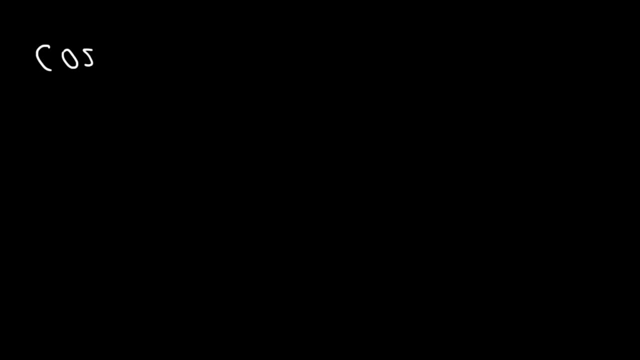 And sine is positive in quadrant 2.. So sine 150 is 1 half. So therefore the exact value of this expression is equal to sine 150, which is equal to 1 half. So that's the answer. Let's work on a similar problem. 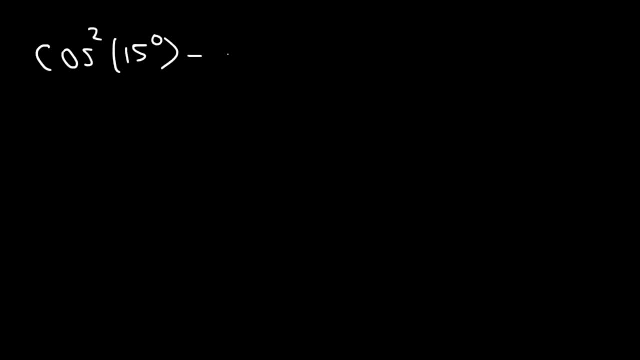 Cosine squared of 15 degrees minus sine squared of 15 degrees. That's equal to what? What is the exact value of that expression? So let's use this formula: Cosine squared theta minus sine squared theta is equal to cosine 2 theta. 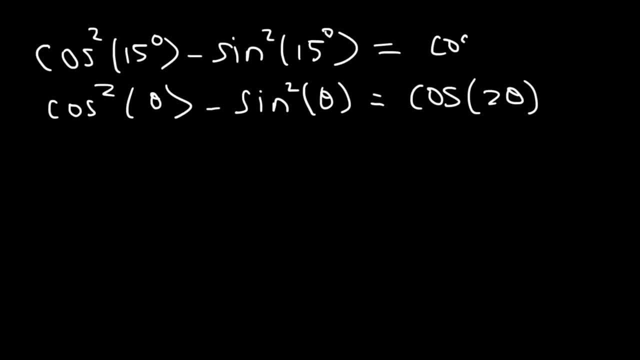 So cosine squared 15 minus sine squared 15 is cosine 2 times 15 degrees, Which is cosine of 30 degrees, And based on the 30-60-90 triangle, Cosine is equal to sine of 30 degrees. Cosine is equal to the adjacent side divided by the hypotenuse using 30 as the angle. 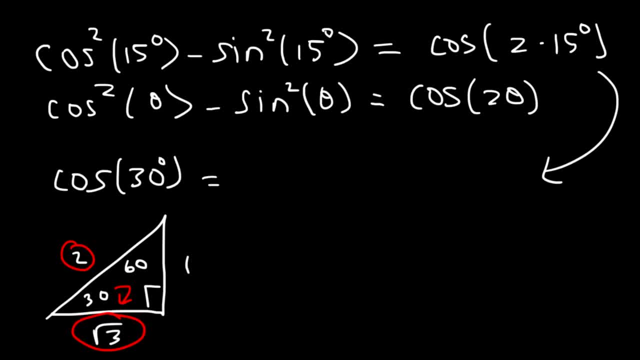 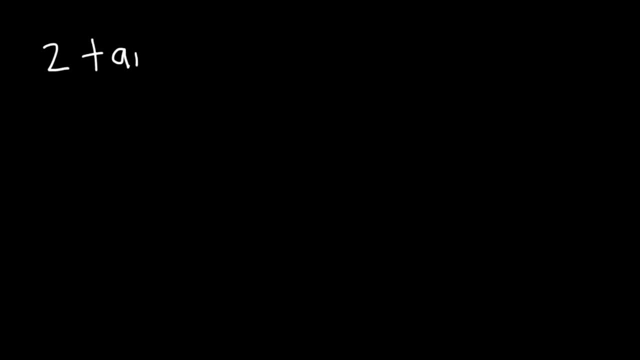 Root 3 is adjacent to 30. So cosine 30 is equal to the square root of 3 divided by 2.. Let's work on one more example. What is the value of 2 tangent of 22.5 degrees divided by 1 minus tan squared of the same? 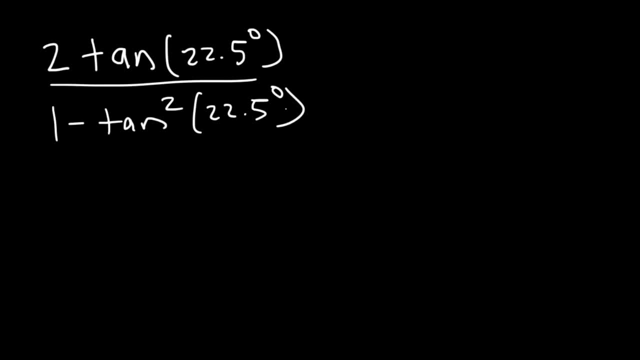 angle, 22.5 degrees. So, using what you know, what's the answer? Well, we can recognize the formula. This is the double angle formula of tangent. So 2 tan over 1 minus tan, squared, that's equal to tangent of 2 theta. So this expression is tangent of 2 times 22.5 degrees.